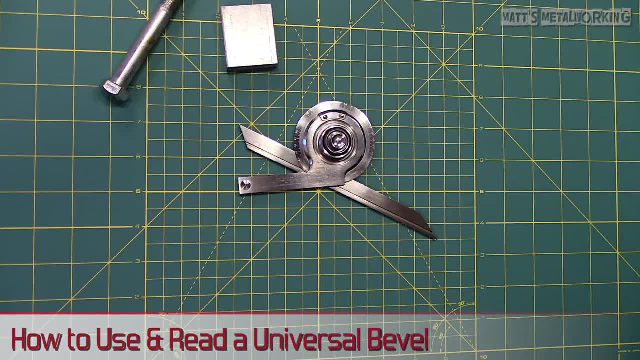 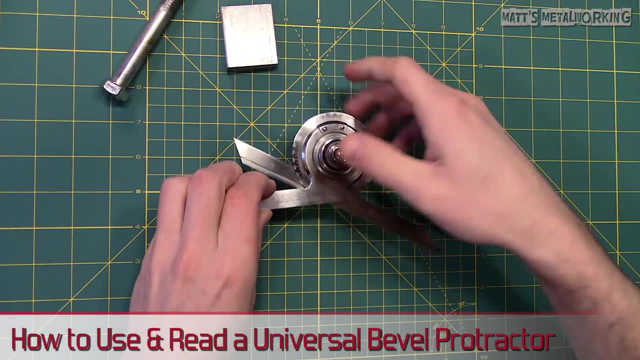 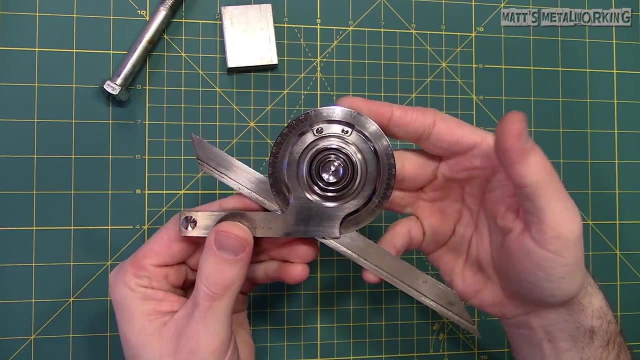 Welcome to another video from Matt's Metalworking. In this video, I will be explaining what is a universal bevel protractor and how to read one. This protractor is a precision gauge used to check angles on parts, which holds an accuracy up to five minutes using the Vernier scale. Some also 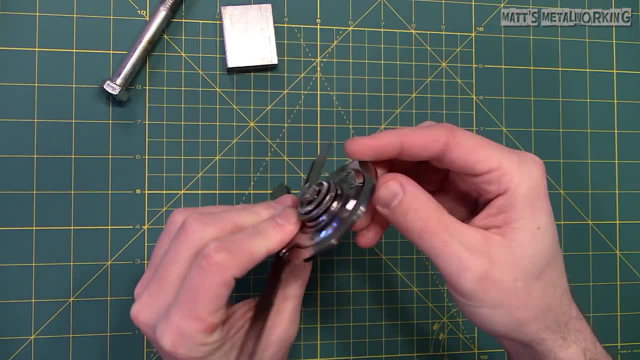 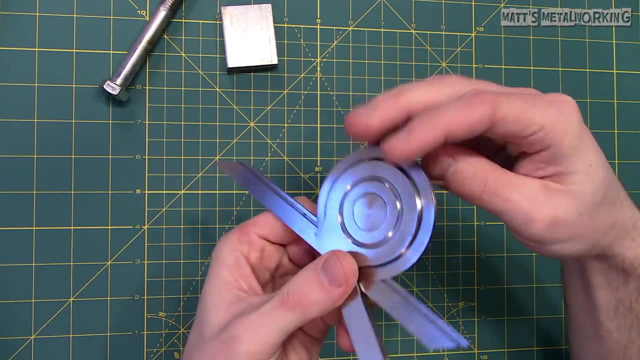 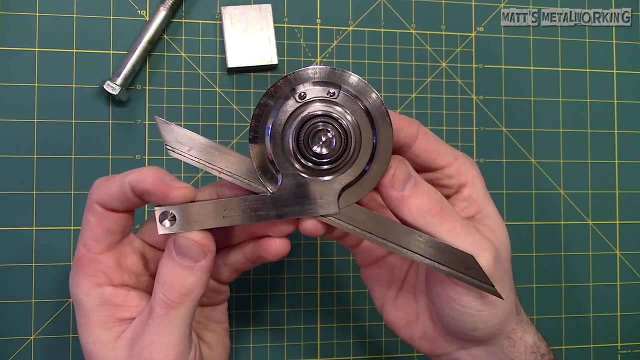 have a magnifying glass over the Vernier scale for easier viewing. How to read a protractor with Vernier scale will be towards the end of the video. It's able to rotate 360 degrees but is broken down into 90 degree segments. It can be read in both clockwise and counterclockwise directions. 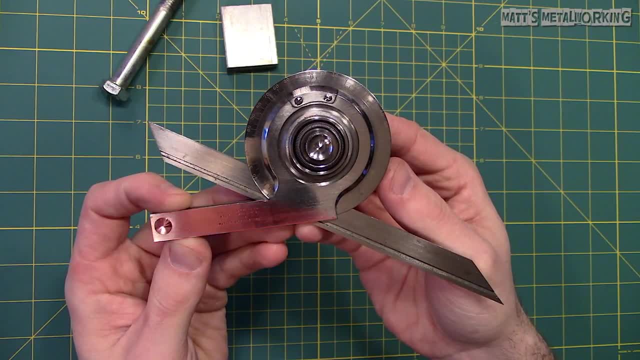 which I'll show you in a moment. First, we have a beam, also known as a base or stock, which is a stationary piece used as a measuring edge. Sometimes you can also mount an acute angle attachment to the beam to measure acute angles. Next is a blade that rotates along with the protractor and can also be adjusted. 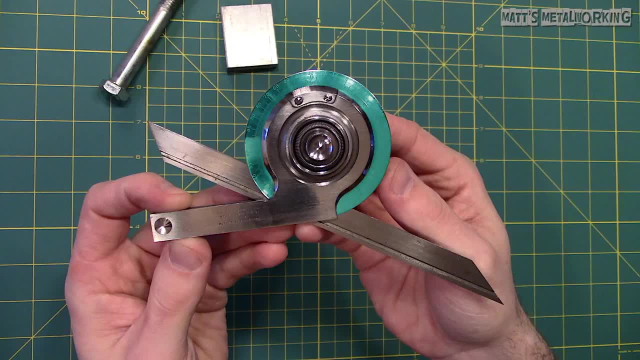 Here's a protractor. as mentioned earlier, it rotates 360 degrees but is broken into 90 degree segments: The lock for the protractor to keep everything in place, Another lock for the blade to prevent it from moving. A fine adjustment that needs to be pushed down to engage gear. so the 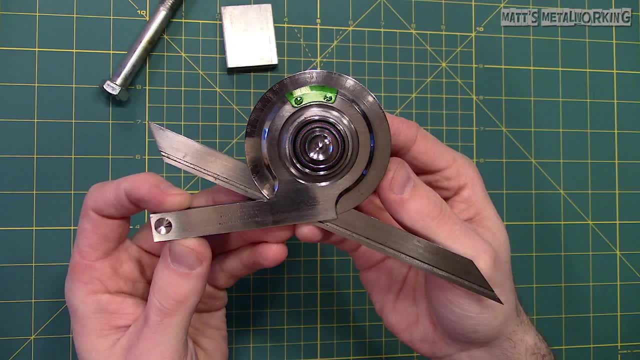 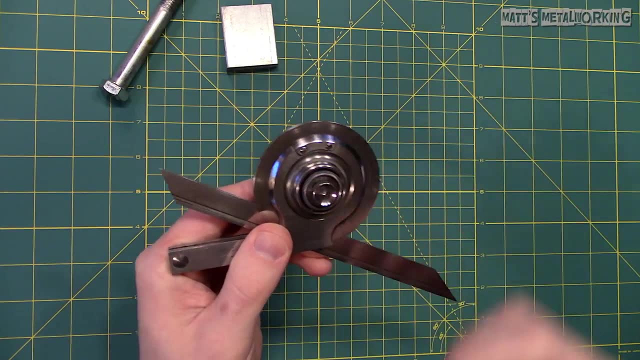 protractor can be moved up and down. Next is a metallock. It's made for set-up and use to set up. batteries can move. and finally, the Vernier scale, allowing us to achieve an accuracy within five minutes. This particular protractor is made by Sterrett Other. 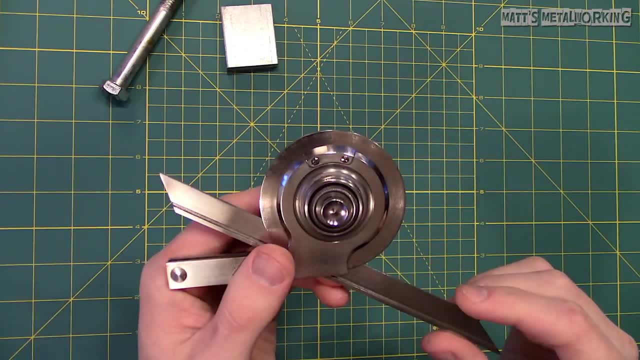 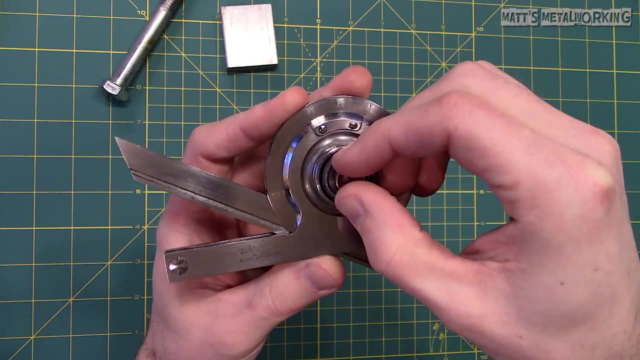 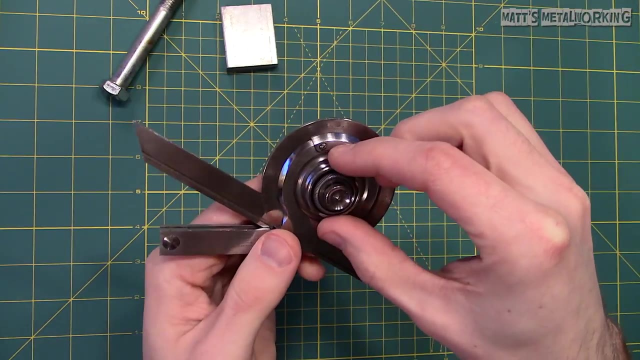 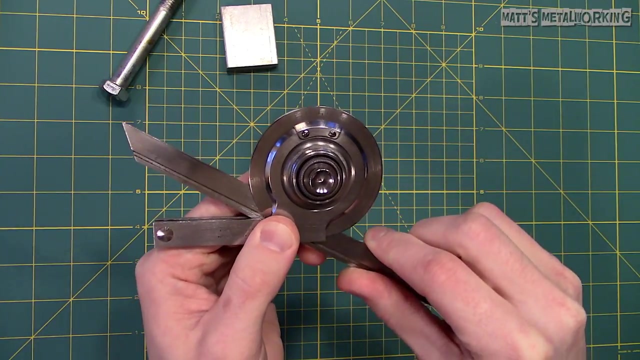 manufacturers are available as well. Styles and qualities will also vary. Now to show you the protractors operations: when the blade lock is disengaged and, as you can see, the blade moves freely, Rotate the lock and the blade is locked into place. Next, disable the protractor lock and it rotates freely. Tighten and 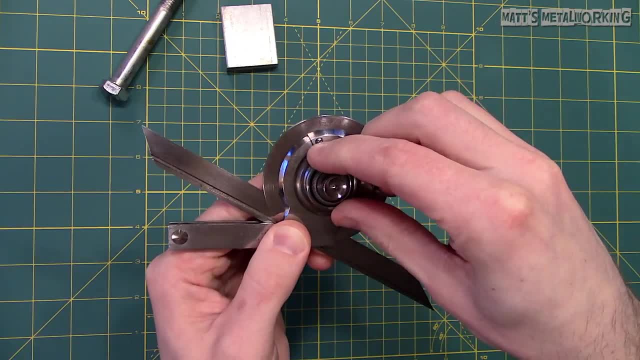 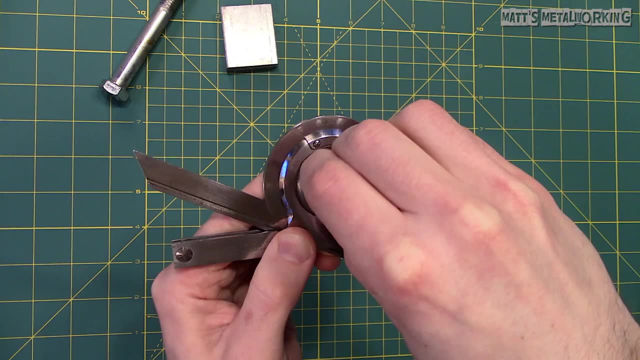 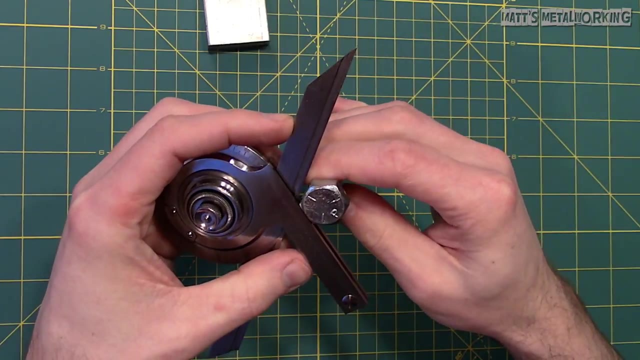 then it's locked into place. Disengage the lock again, Then push down the fine adjustment to engage the gear and twist to rotate the protractor. Now to measure the bolt head, demonstrating the protractor can measure from either side of the beam. Ensure the blade is locked so it doesn't have any movement, or 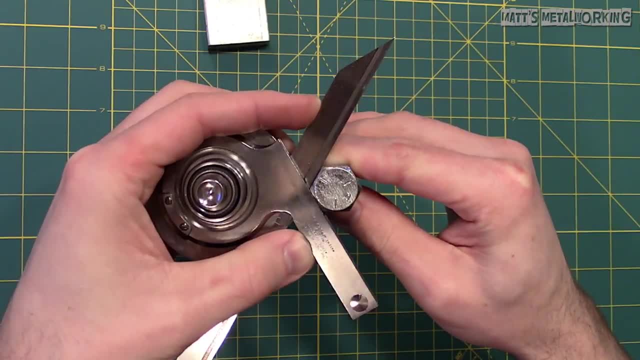 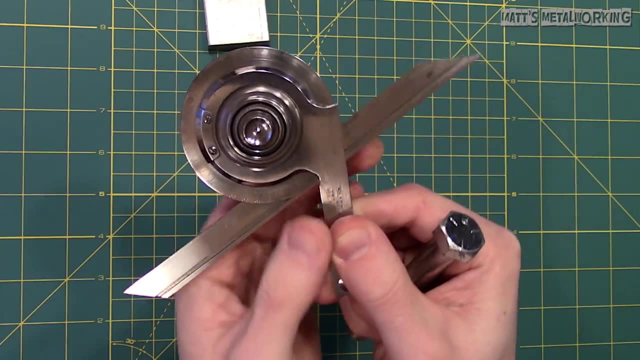 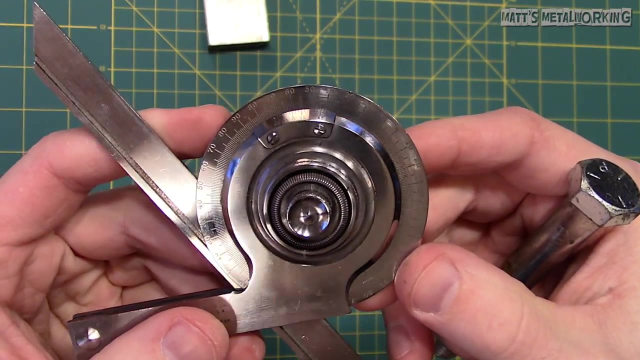 damage. Push the object against the working edge and align the blade against the other surface, Lock the protractor and take the reading. We have a reading of about 60 degrees and we are measuring in a counterclockwise direction In order to calculate over a 90 degree angle, which we have minus your reading from. 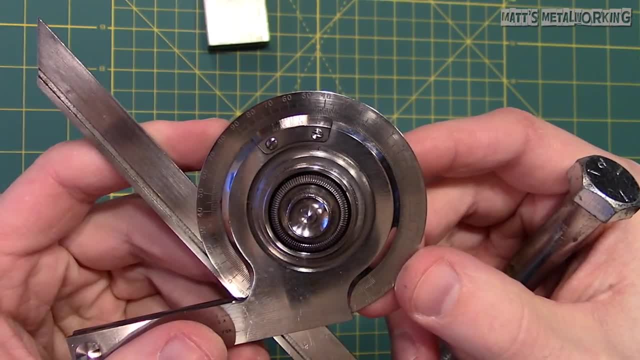 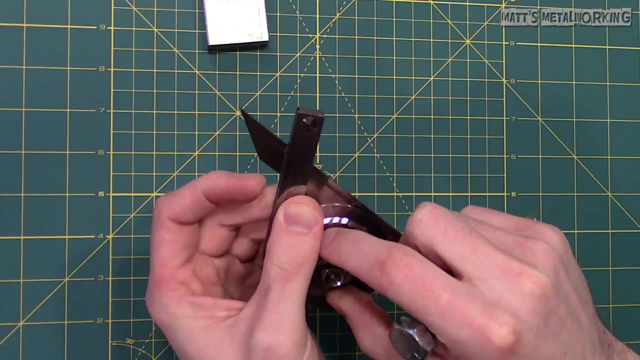 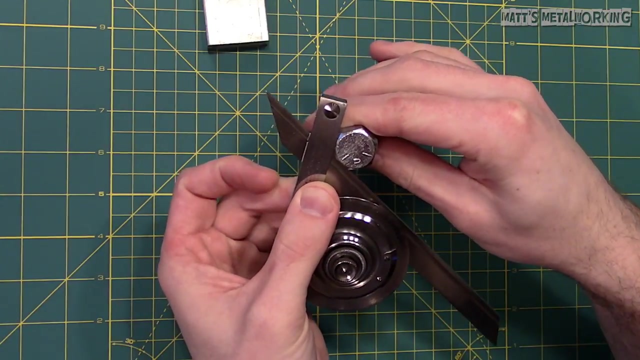 180. this gives us 120 degrees. In a moment, I'll show you how to use the Vernier scale. We are going to put the bolt on the beam again. this time the opposite side. Here we are measuring in a clockwise direction. therefore, the numbers are increasing to the right With 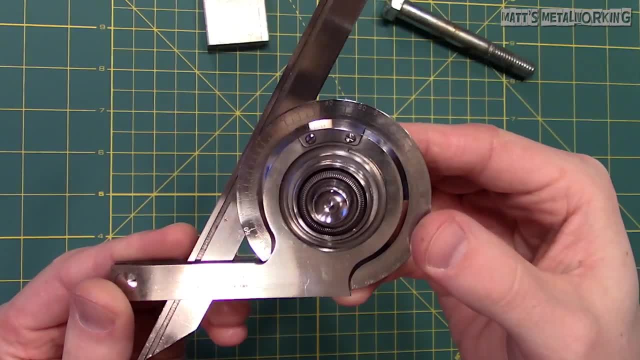 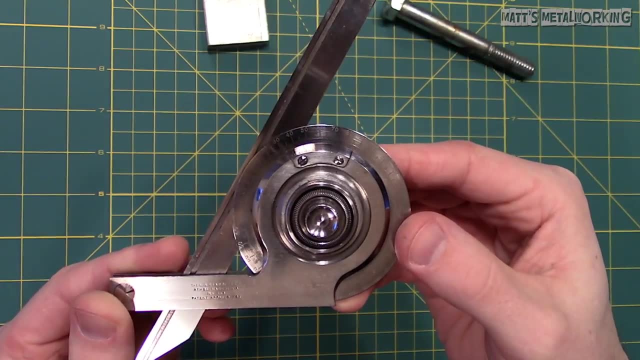 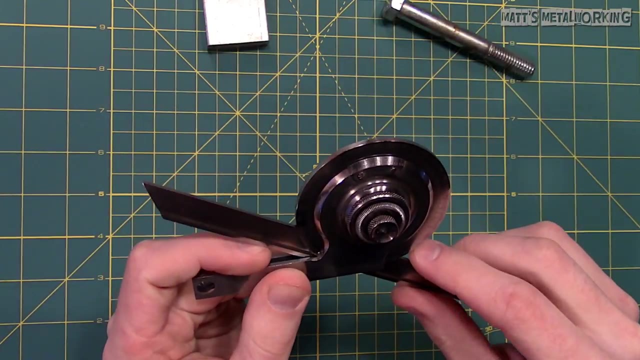 the reading of 60 degrees. measuring an angle greater than 90 degrees, 180 minus 60 gives us a final measurement of 120 degrees. Moving on to reading the Vernier scale, just setting the bevel protractor on a random reading. while this can be harder to see on camera due to 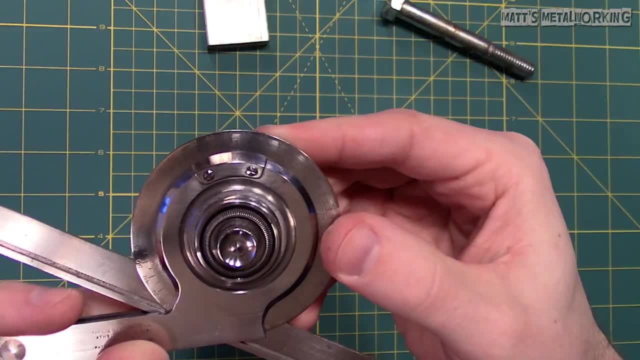 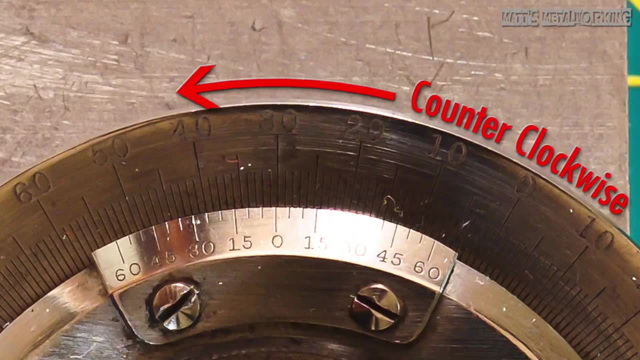 the glare. I have taken extra photos for a better visual representation. As you can see, the numbers are increasing in the counterclockwise direction. Taking the first reading using the zero line on the Vernier scale, which line does it pass on the protractor First? we have 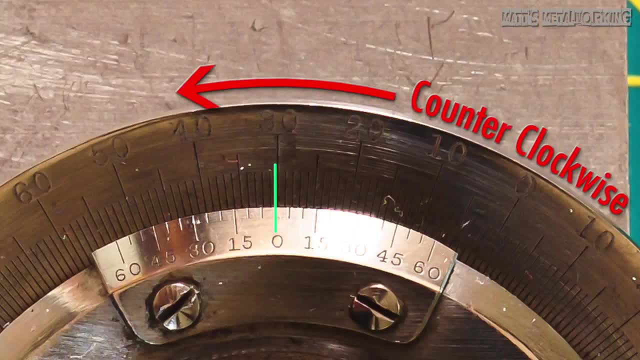 30 degrees. Considering we are travelling in the counterclockwise direction, the Vernier scale must go in the same direction. Determine which line between the Vernier scale and protractor aligns best. This would be 25 minutes. The final result would be a 30 degrees 25 minutes. 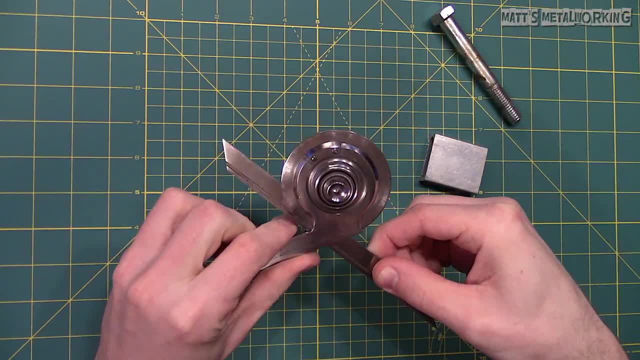 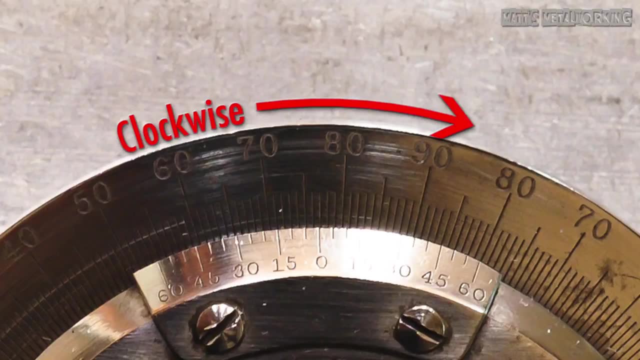 measurement. The next example, this time measuring in a clockwise direction- again determine which line the zero on the Vernier scale passes on the protractor. This time it's 76 degrees. which line does the protractor and Vernier scale align with best, Being that we are travelling in the clockwise? 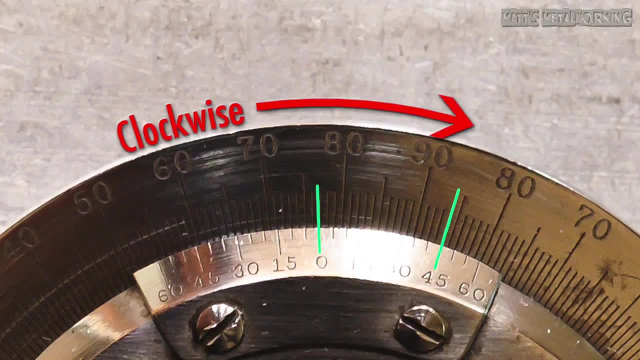 direction. This time it's 76 degrees. Which line does the protractor and Vernier scale align? do the same with the Vernier scale. We have 45 minutes, 76 degrees and 45 minutes is our final measurement. And a third example, Traveling in the clockwise direction: the zero line on the Vernier.